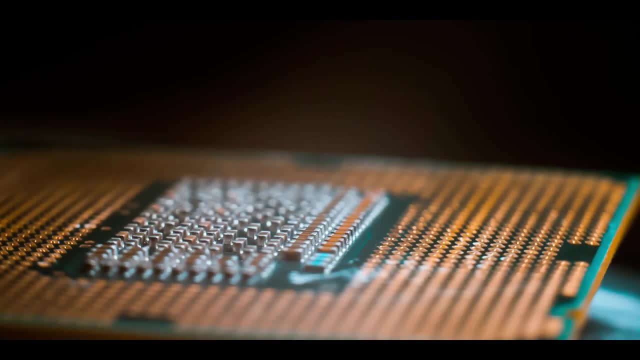 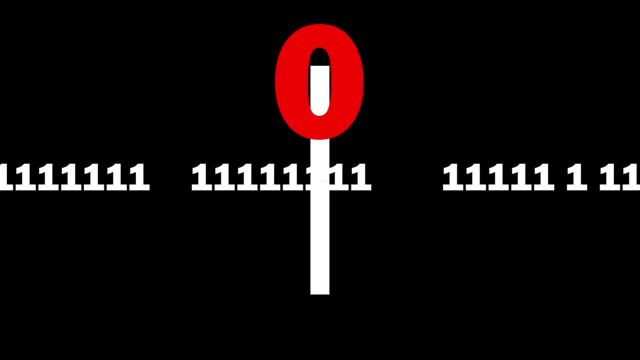 But computers are getting super duper small, to the point where the size of computer opponents isn't too far from the size of an atom. This is a problem because once you get small enough, the laws of physics change and electrons will just go through the switch wall anyway, giving no fricks. 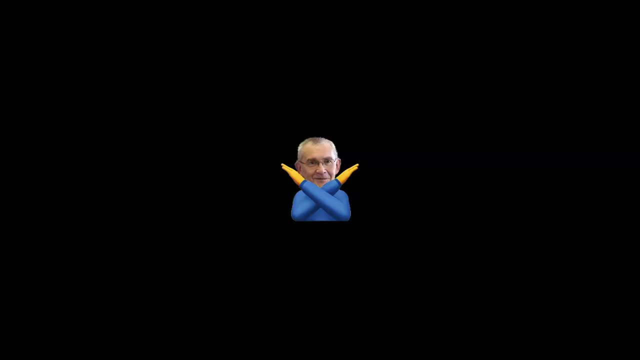 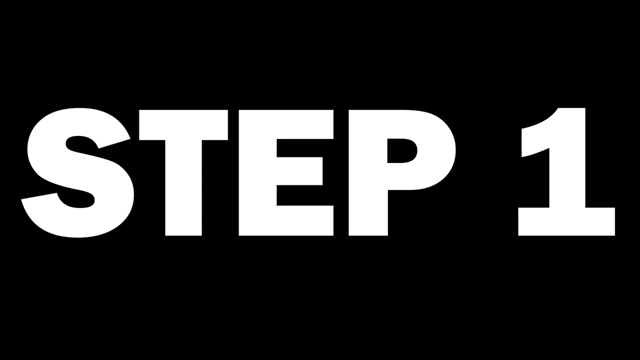 thank you. quantum tunneling: Cool. so computers just won't get any better. No, said some nerd probably. What if we just use this weird quantum stuff to our advantage? So he made a quantum computer. Now you will too, with this guide. Step one: make a qubit. Cubits are the bits. 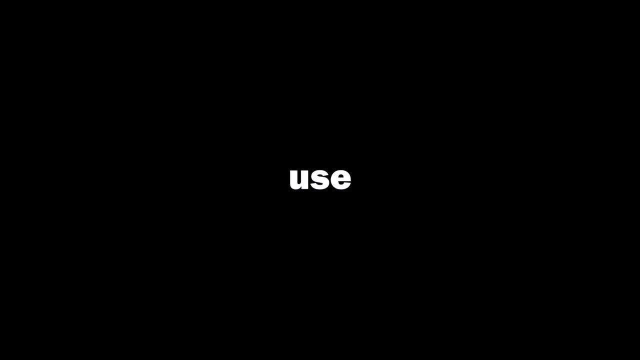 of quantum computers just way cooler. Cubits don't use electrons like a normie. instead they use other stuff like photons or magnetic field spinning. Thanks to this, qubits can represent not just one or zero, but it makes it both in any proportion. Congratulations. now you have a superposition. 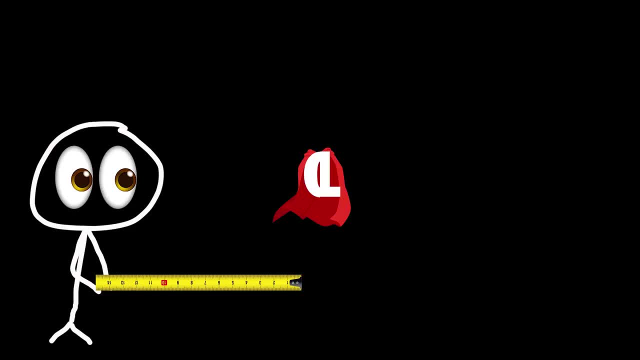 qubit. Step two: manipulate superposition qubit. Oddly, whenever you look at or measure a superposition, it makes up its mind and takes one definitive side. Why, you ask? I don't know, I just got here. Anyways, these superposition qubits can store like way more information than your average bit. 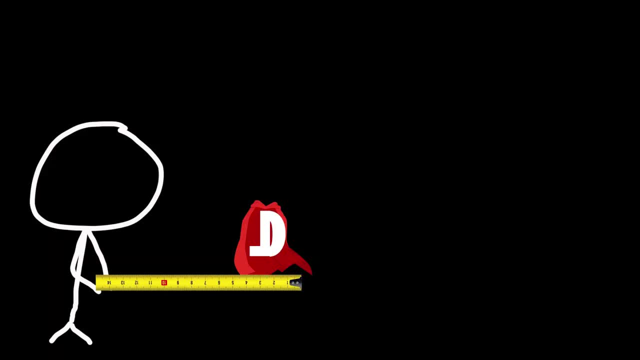 Also, these qubits are intertwine dizzled, no matter how far apart they are, so if you measure one of them you can pretty much predict the other. We just need to make a gate to manipulate this simulator irregular computer just way, way, way harder. You're going to need a quantum gate. You probably don't. 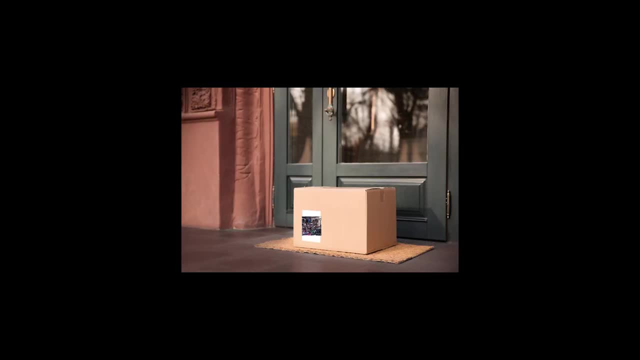 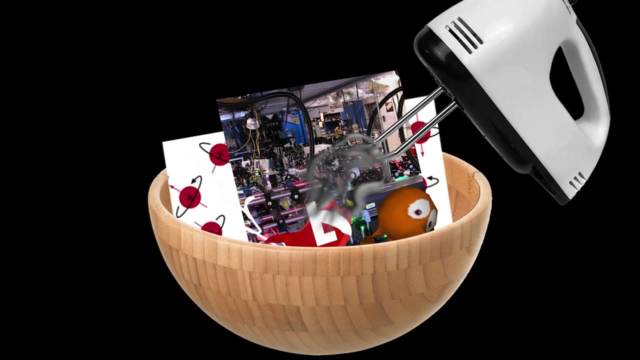 have one lying around, but you should be able to find one on ebay for relatively cheap. Once you have one, get a superposition in the gate, takes note of it, it throws another superposition out and you're all good to go. Step three: put it all together and mix. Flip the on button to your new. 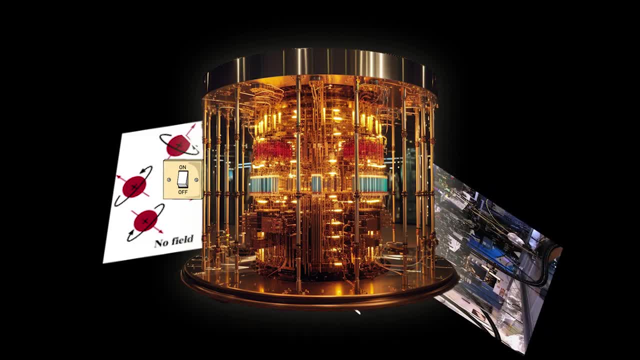 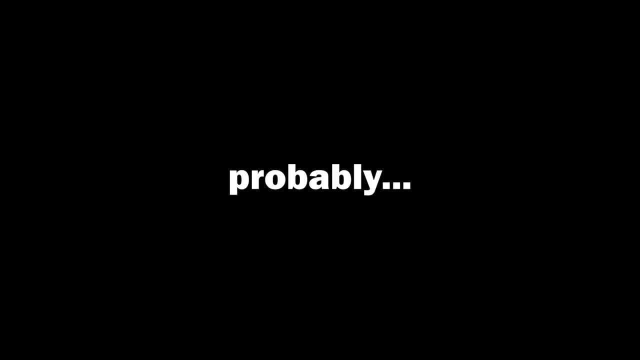 quantum computer. It will manipulate some probabilities and after that measure an outcome, observing the superpositions as actual ones and zeros. Step four: what to do with your new quantum computer. They won't replace your phone or computer, Probably, But it would be really good. 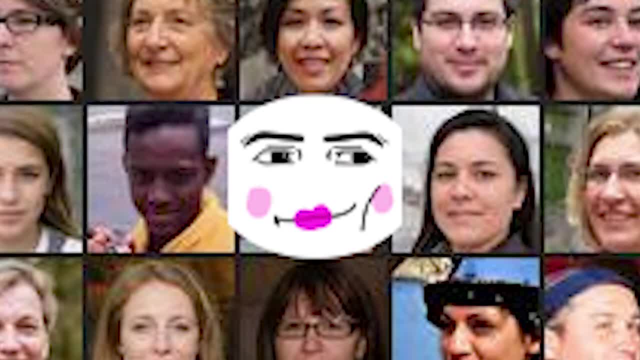 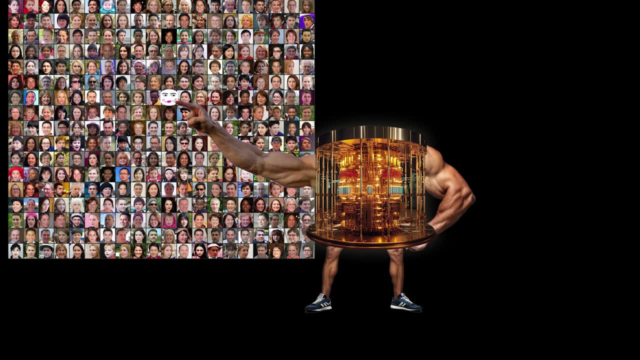 at finding stuff. Imagine you ask a regular computer to find a picture of your mom in a database of billions of moms. Your computer would have to test every single mom. But a quantum computer would find your mom insanely fast, Not just because she's morbidly obese, but also because 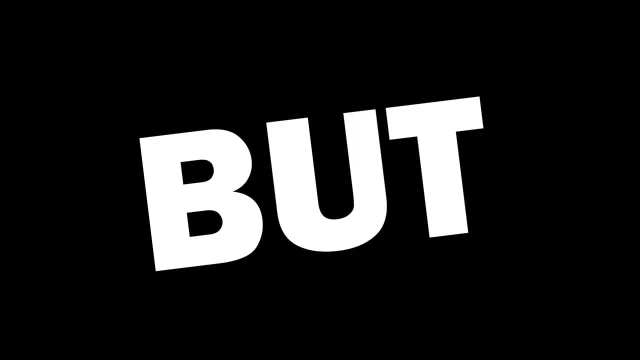 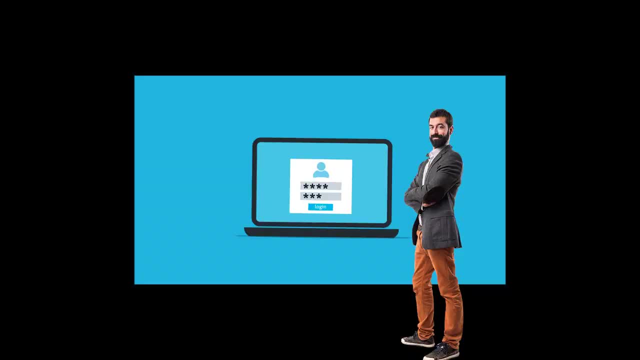 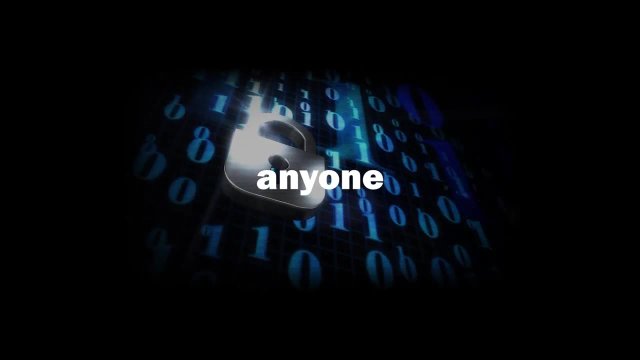 it can process the information way faster thanks to superpositions. But even better than that, your quantum computer will be really really good at absolutely destroying IT security. Say you want all of your best friend's data. Well, your best friend's data and passwords is kept secure through an encryption system with a public key that anyone could get to. 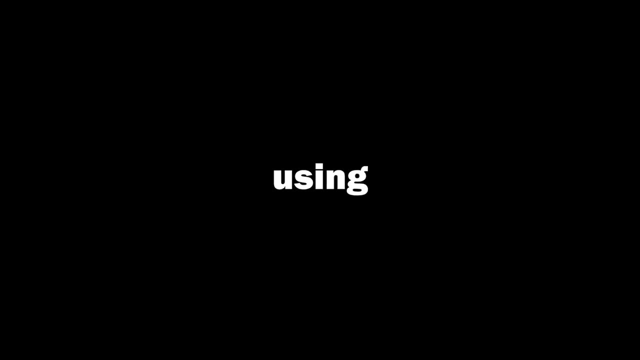 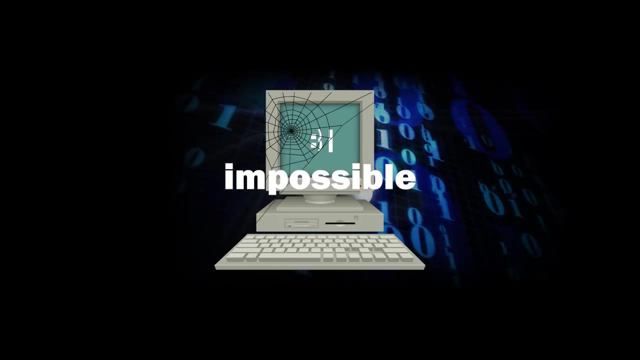 Luckily, only your best friend can decode them. But technically, using reverse engineering, you could use this public key to steal all your best friend's goodies. Using a regular computer, this would take years and is pretty much impossible. With your new quantum computer, you could do this.